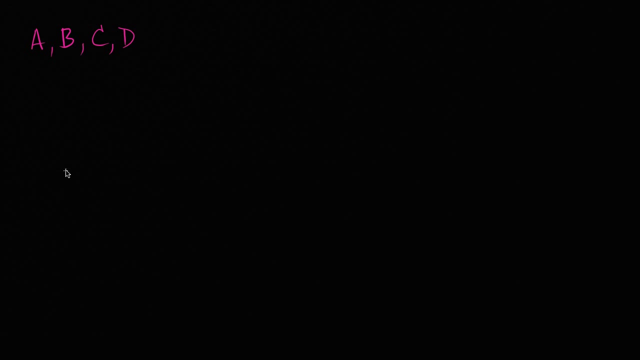 All right, I'm assuming you've had a go at it, So one way to think about it is okay. if you say there's a handshake, well, a handshake has two people are party to a handshake. We're not talking about some new three-person handshake. 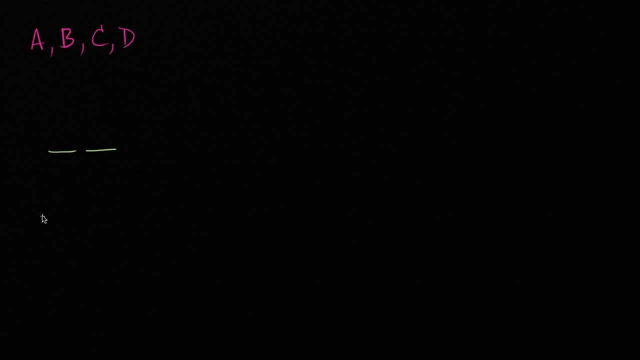 or four-person handshake. We're just talking about the traditional. two people shake their right hands, And so there's one person and there's another person that's party to it, and so you say: okay, there's four possibilities of one party. 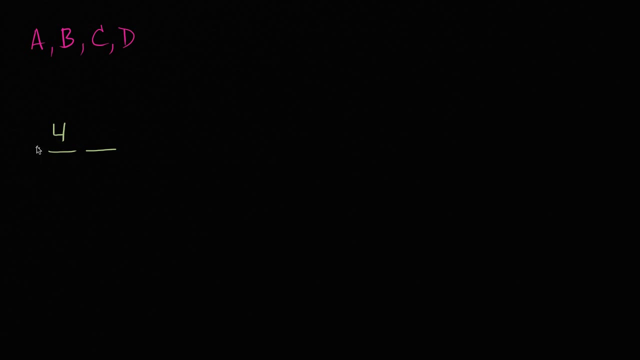 and if we assume people aren't shaking their own hands- which we are assuming, where they're always gonna shake someone else's hand- then for the other party there's only three other for each of these four possibilities. who's this party? 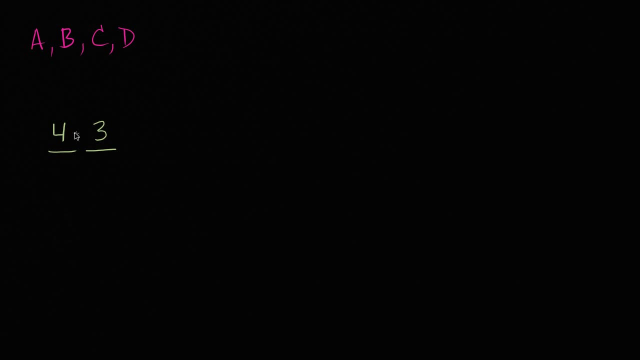 there's three possibilities. who's the other party? And so you might say that there's four times three handshakes. Since there's four times three, I guess you could say possible handshakes, And what I'd like you to do is think a little bit about. 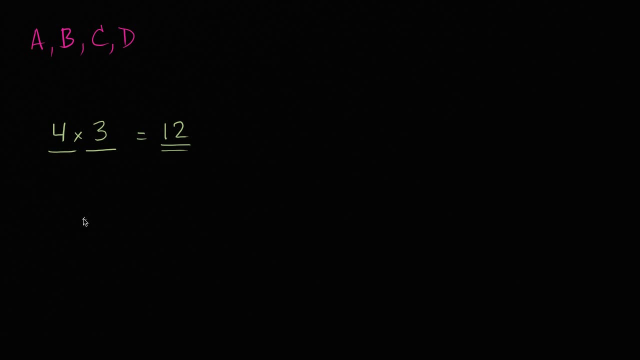 whether this is right, whether there would actually be 12 handshakes. Well, you might have thought about it and you might say: well, you know this, four times three, this would count. this is actually counting the permutations. 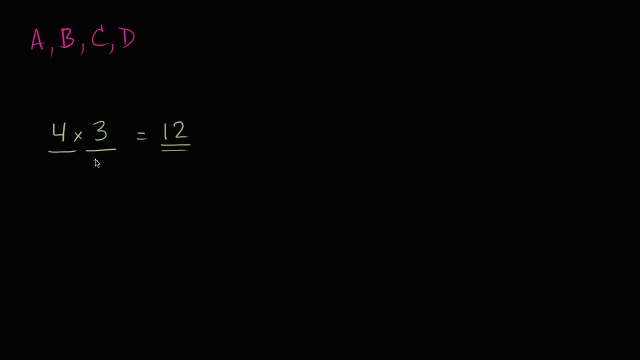 This is counting. how many ways can you permute four people into two buckets, the two buckets of handshakers, where you care about which bucket they are in, whether they're their handshaker number one or handshaker number two? This would count. this would count, A being the number one. 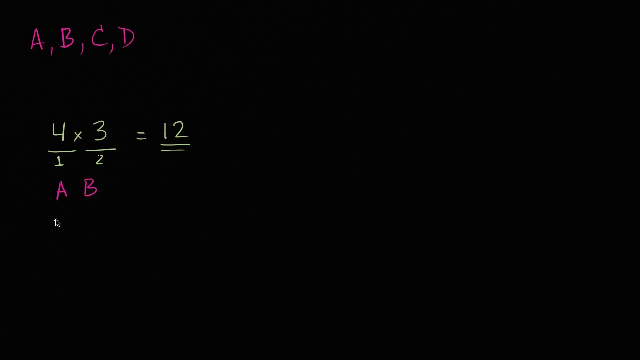 handshaker and B being the number two handshaker, as being different than B being the number one handshaker and A being the number two handshaker. But we don't want both of these things to occur. We don't want A to shake B's hand where A is facing north. 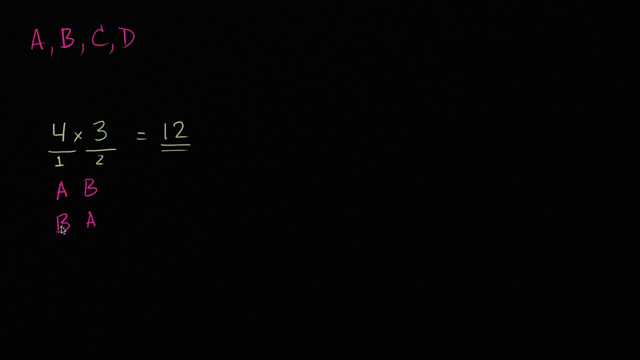 and B is facing south, and then another time they need to shake hands again where now B is facing north and A is facing south. We only have to do it once. These are actually the same thing, so no reason for both of these to occur. 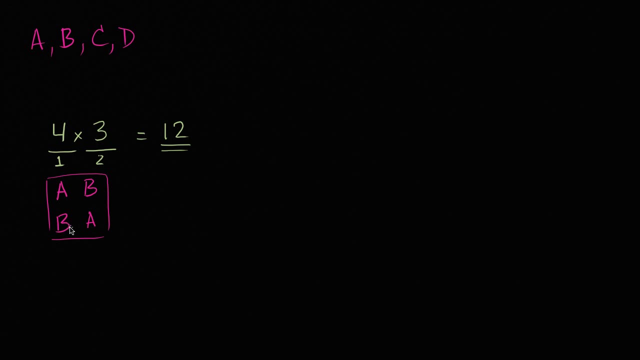 So we are going to be double counting. So what we really want to do is think about combinations. One way to think about it is: you have four people In a world of four people, or a pool of four people. how many ways can you choose two? 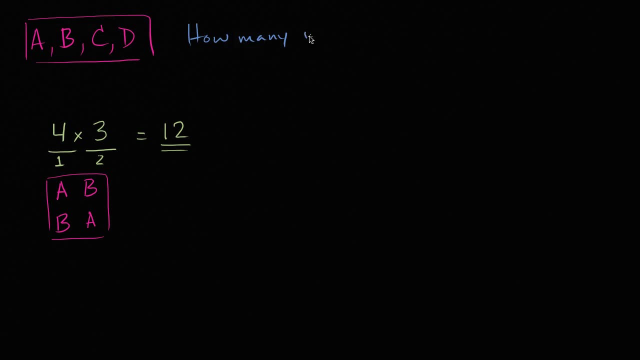 How many ways to choose two, Because that's what we're doing. Each handshake is just really a selection of two of these people, And so we want to say how many ways can we select two people so that we have a different each combination? 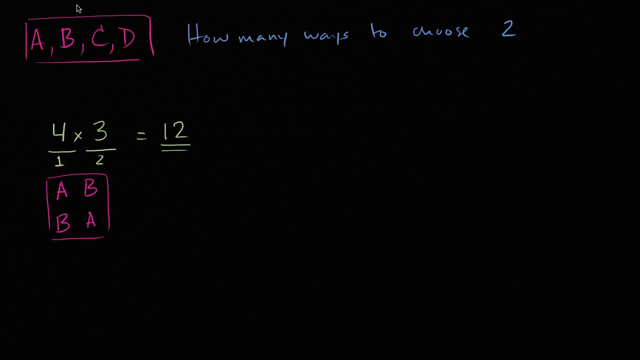 each of these ways to select two people should have a different combination of people in it. If two of them had the same- A, B and B A- these are the same combination, And so this is really a combinations problem. This is really equivalent to saying how many ways. 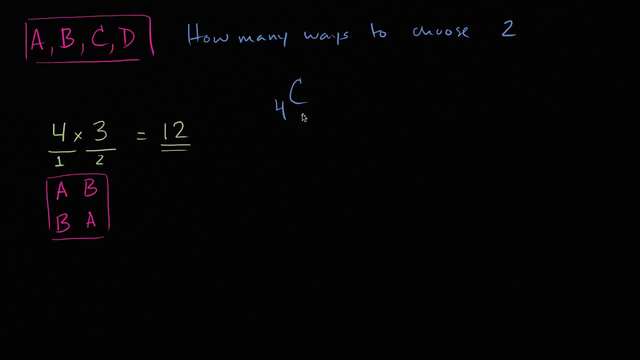 are there to choose two. How many ways are there to choose two people from a pool of four, Or four choose two, Or four choose two. And so this is going to be well. how many ways are there to permute four people into three spots? 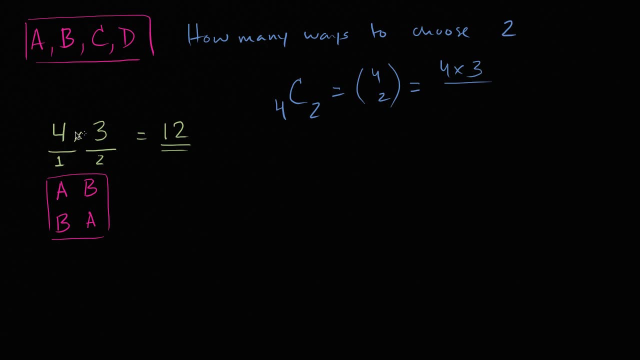 Which is going to be four times three, which we just figured out right over there, which is 12.. I actually want to do it in that green color, so you see where that came from. So four times three. So you're going to divide that by the number of ways. 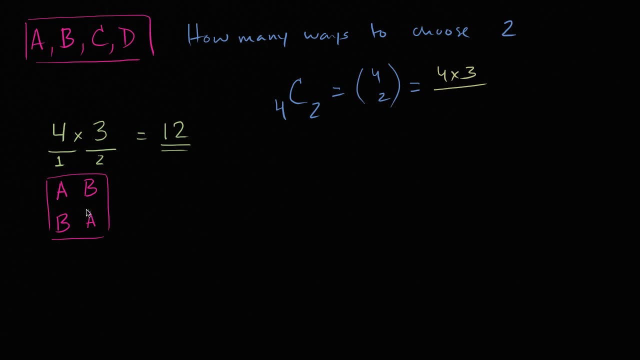 you can arrange two people. Well, you can arrange two people in two different ways: One's on the left, one's on the right, or the other one's on the left and the other one's on the right, Or you could also view that as two factorial. 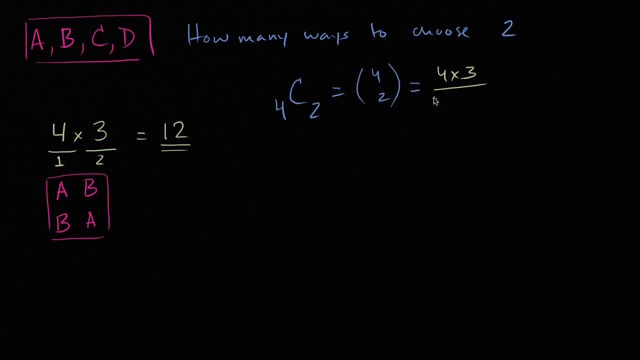 which is also equal to two, So we could write this down as two. So this is the number of ways to arrange two people, Two people, Two people, And this up here. this up here is, let me just in a new color. 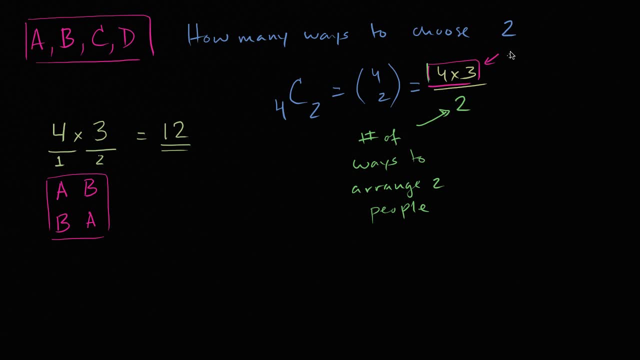 this up here. that's the permutations, That's the way number of permutations if you take two people from a pool of four. So here you would care about order, And so one way to think about it, this two is correcting for this double counting here. 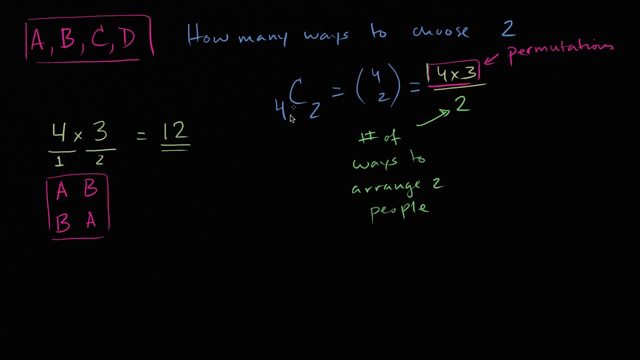 And if you wanted to apply the formula, you could. I just kind of reasoned through it again. I mean you could literally say: okay, four times three is 12.. We're double counting because there's two ways to arrange two people. 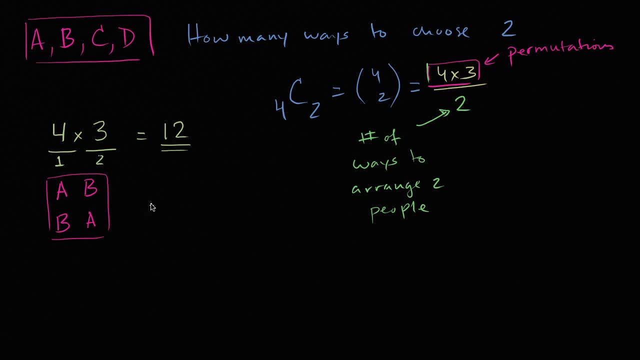 So you just divided it by two. So you just divide by two, And then you are going to be left with six. You could think of it in terms of this, Or you could just apply the formula. You could just say: hey look. 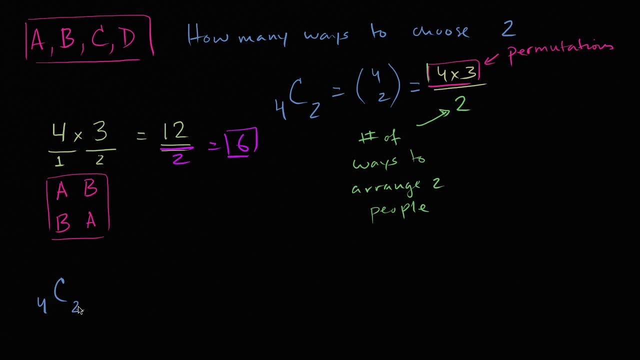 four. choose two, or the number of combinations of selecting two from a group of four. This is going to be four factorial over two factorial times, four minus two. Four minus two factorial, And let me make this color different, just so you can keep track of. 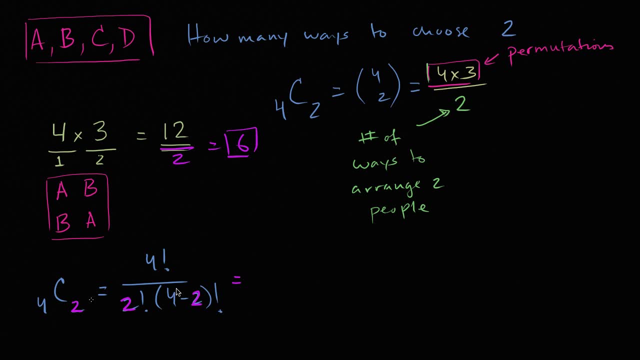 how I'm at least applying this. And so what is this going to be? This is going to be four times three times two times one, over two times one times this right over here is two times one, So that will cancel with that. Four divided by two is two. 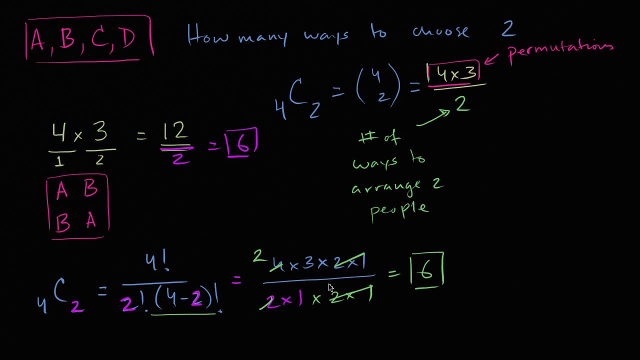 Times three divided by one is equal to six. And to just really hit the point home, let's actually draw it out. Let's draw it out So: A could shake B's hand, A could shake C's hand, A could shake D's hand. 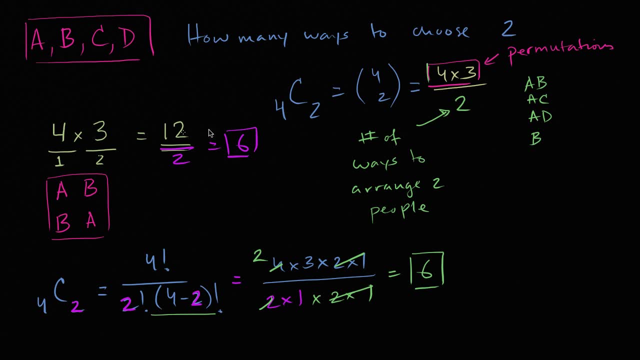 Or B could shake. and let me just do what we calculated first the twelve. We could say: B could shake A's hand. B could shake C's hand. B could shake whoops. B could shake D's hand. We could say C could shake A's hand. 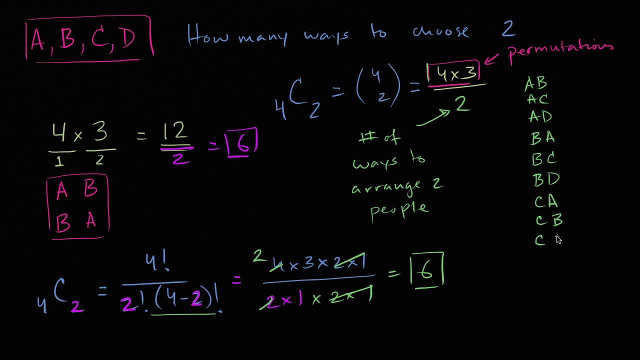 C could shake B's hand, C could shake D's hand. And you could say: D could shake A's hand, D could shake B's hand, D could shake C's hand. And this is twelve right over here, And this is the permutations. 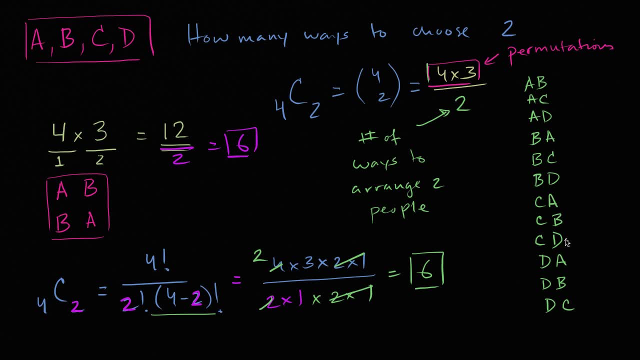 If D shaking C's hand was actually different than C shaking D's hand, then we would count twelve. But we just wanted to say, well, how many ways they just have to meet each other once, And so we're double counting. So AB is the same thing as BA. 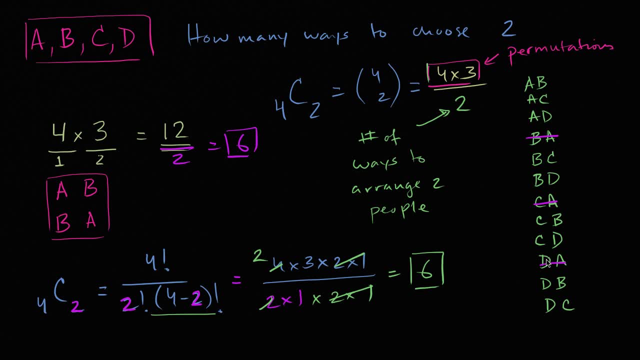 AC is the same thing as CA, AD is the same thing as DA, BC is the same thing as CB, BD is the same thing as DB, CD is the same thing as DC, And so we'd be left with if we correct for the double counting.